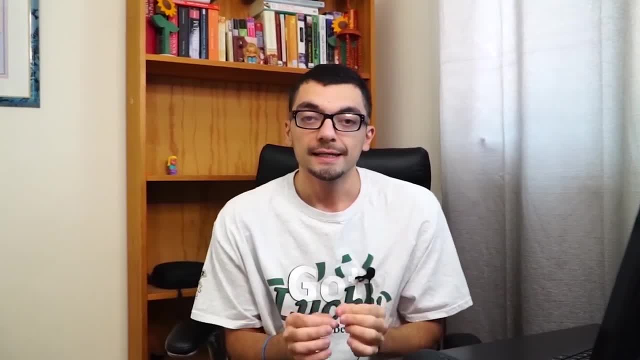 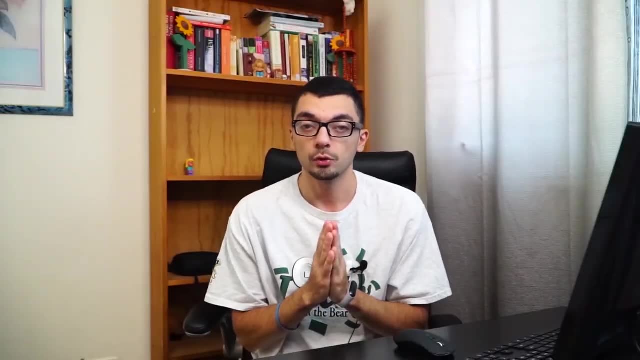 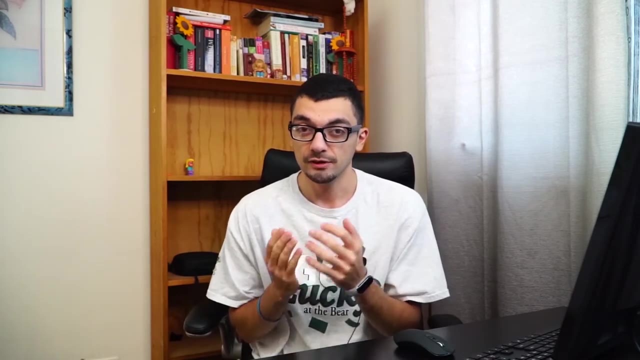 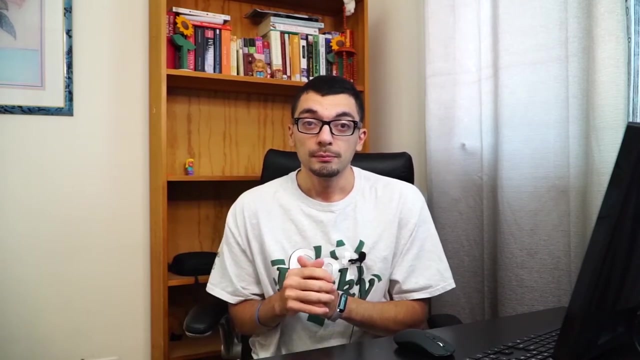 information with different fields and specific topics for the advancement of your research topic. Why it is important? because if you choose outdated topics for doing research or writing your thesis and after graduating your degree, you cannot find and research degrees easily or the job positions in any companies, and that's why I want to help you. 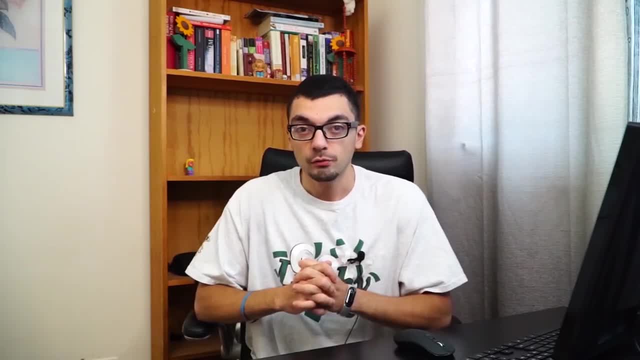 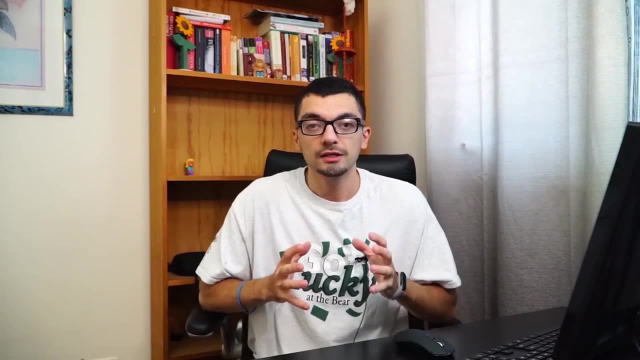 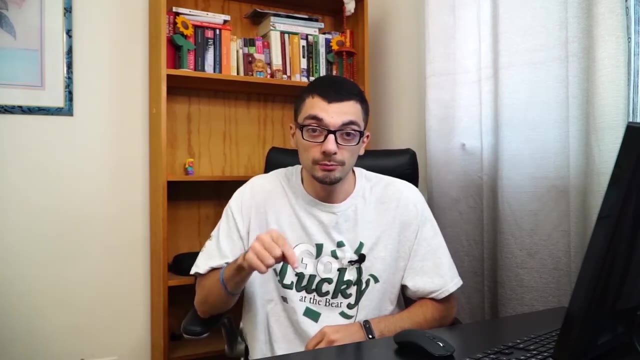 choose trend topics which can apply next five or ten years, even preparing yourself to 2050 year. And today's field? I'm going to start with chemical engineering. If you want me to make videos for your field, comment below, then the next video I will prepare for your field. Let's start Okay. 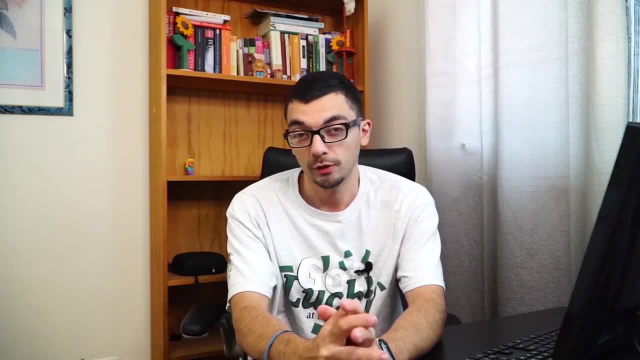 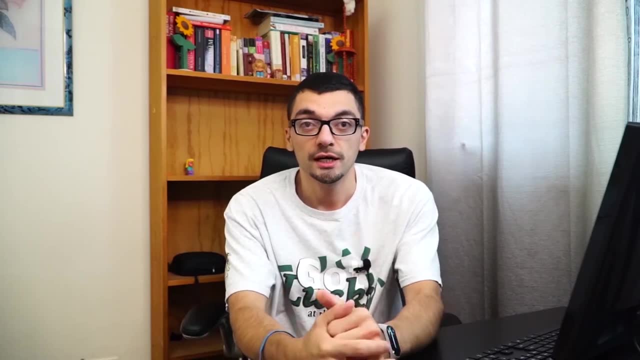 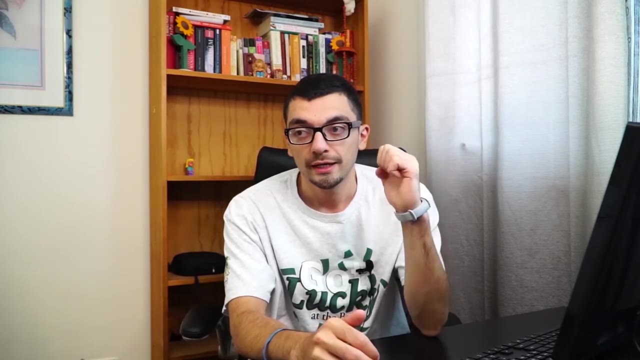 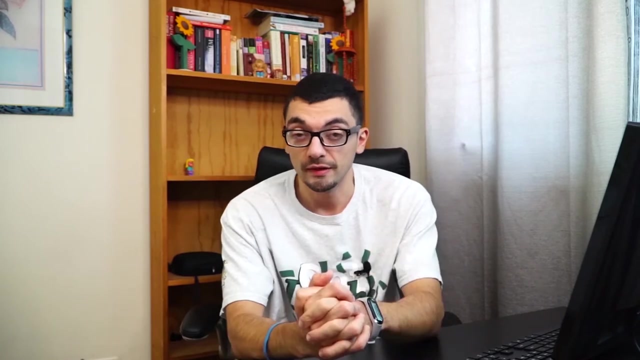 with your chemical engineering degree which topic you can choose in order making your research and job applications perspective in the future. When I can give you the reference bioengineering and health, This is the section of your chemical engineering field and the different departments are taking for this field. If you are talking about bioengineering and health science, first bio. 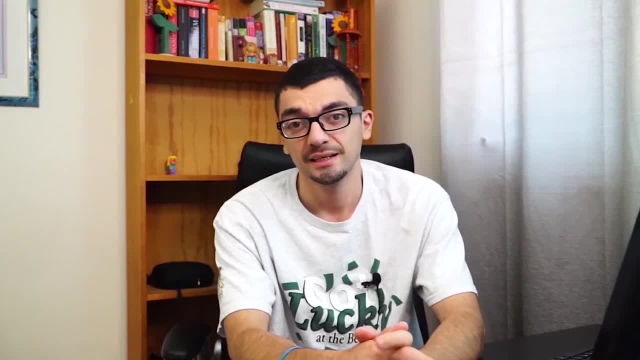 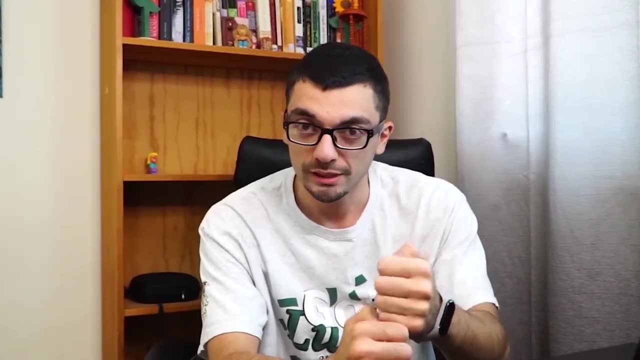 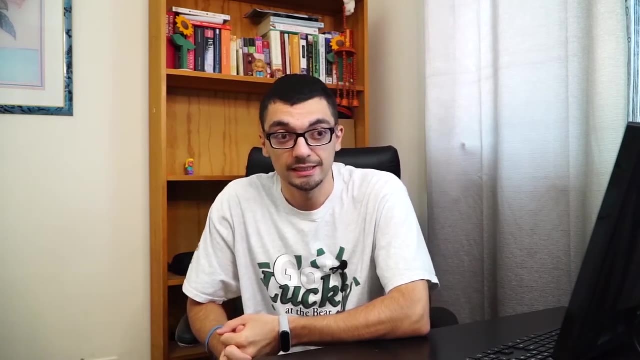 organic chemistry or protein designing, protein modeling, improving biodegradability or biocompatibility of proteins, as well as polysaccharides. This is really effective topics for your research or master thesis After graduating, where you can apply with this topic knowledge, of course, drug industry. 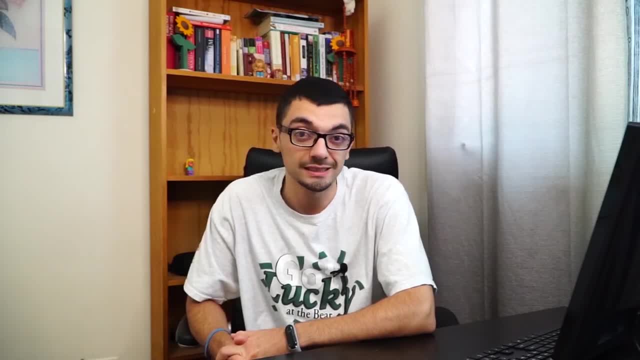 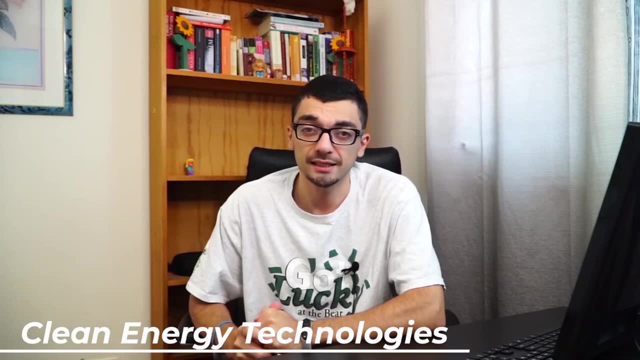 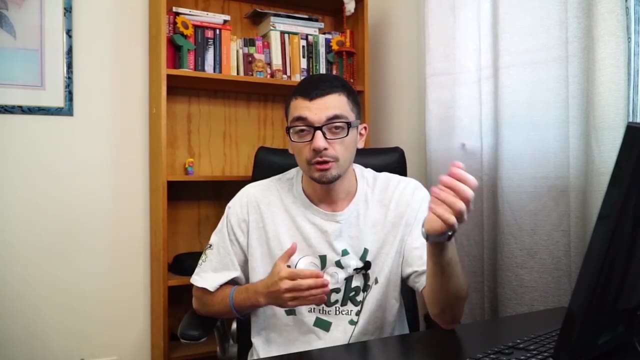 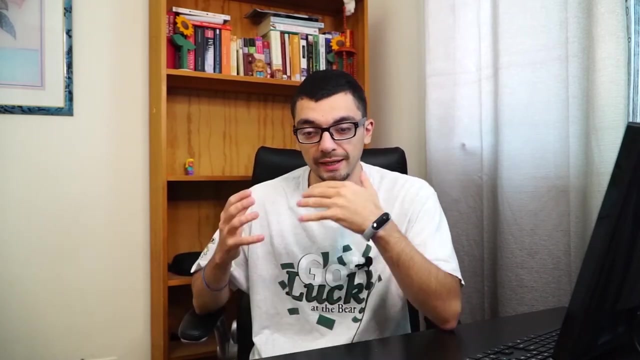 or you can find something related to lung disease or property improvement of liquid metals. This is the first one, and let's go to the second one: clean energy technologies. You can choose several topics related to electrical engineering, power engineering, as well as physical engineering, Chemical engineering and chemistry. that's why the for mixing all of them together and make 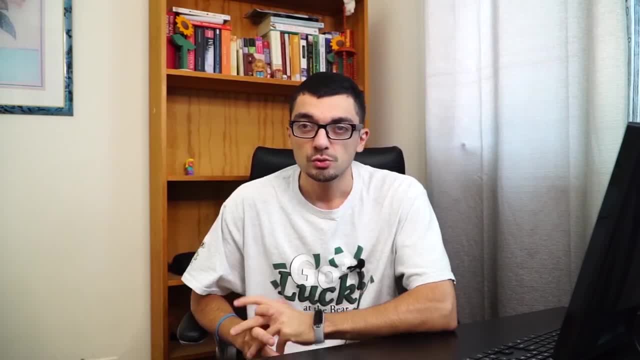 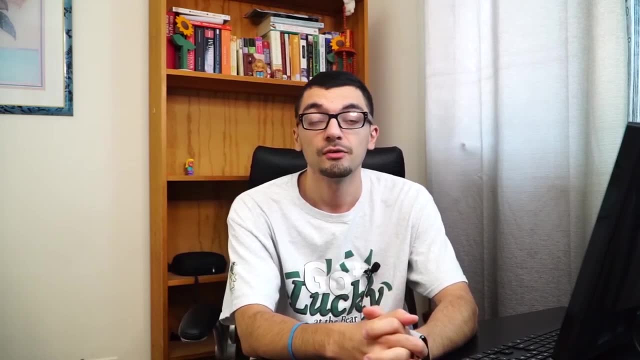 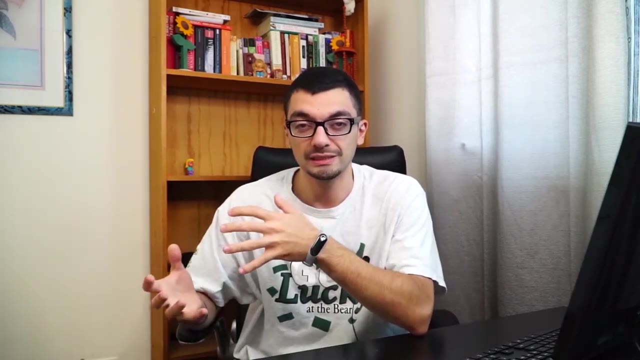 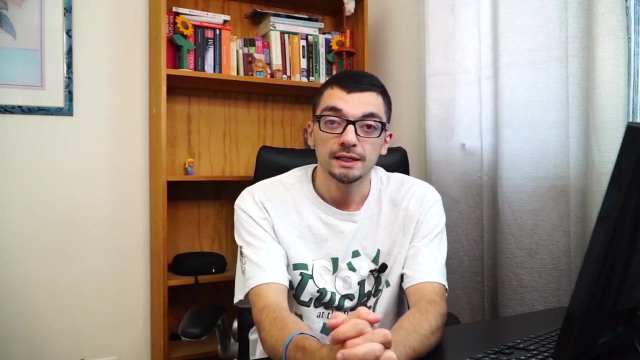 the best research topic for you. You can choose these mentioned topics. first one is kinetics of electrochemical energy conversion. What do I mean? if you are not familiar this topic, this is basically related to chemical properties of electrical materials. These can be combined with various other topics of electrical energy conversion. This is a whole different research. 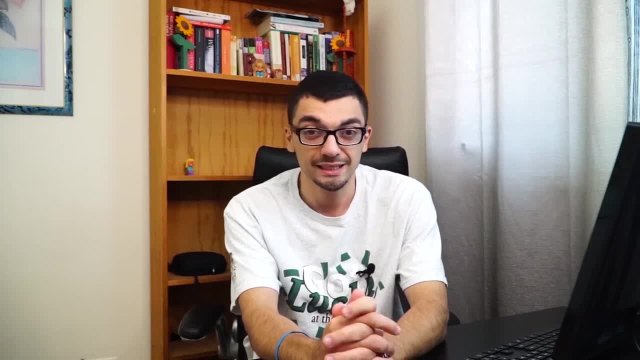 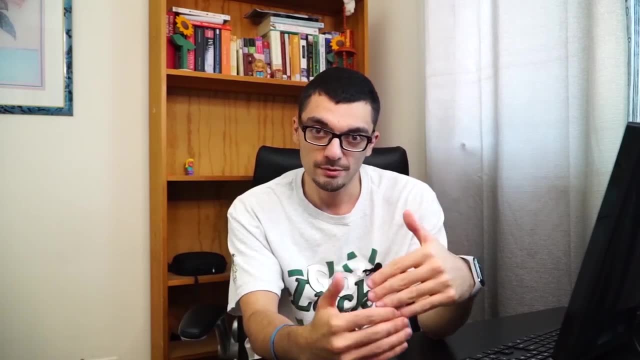 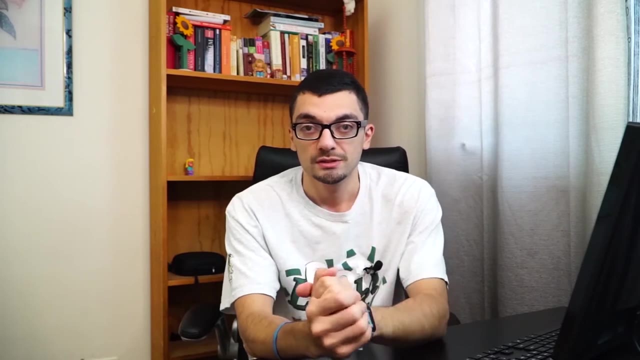 topic for you and another one: advanced battery nanotechnology. We know that lithium batteries and ionization is really dangerous for our environment. You have to find the better solution: how to reduce the damage of these materials and making something less dangerous and environmental friendly batteries for electrical devices. And another one is renewable energy utilization. 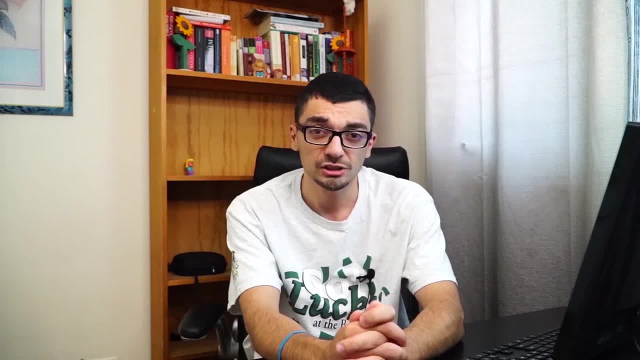 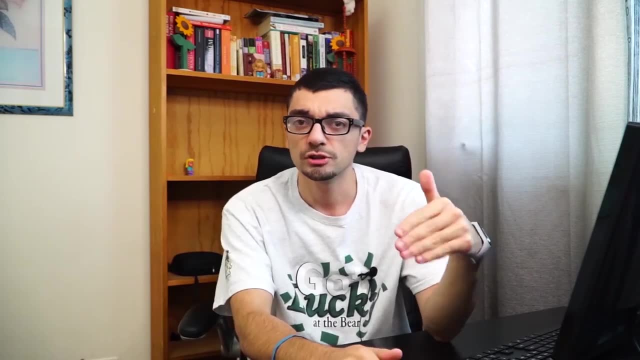 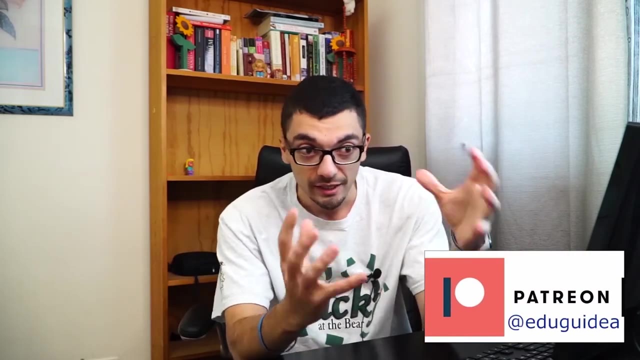 for direct approach to carbon dioxide reduction for sustainable field. yes, this is really a good research topic for you to do research. step by step you will get familiar and you will find some other related topics of these mentioned. it's not really important directly to choose this topic, but something around these. 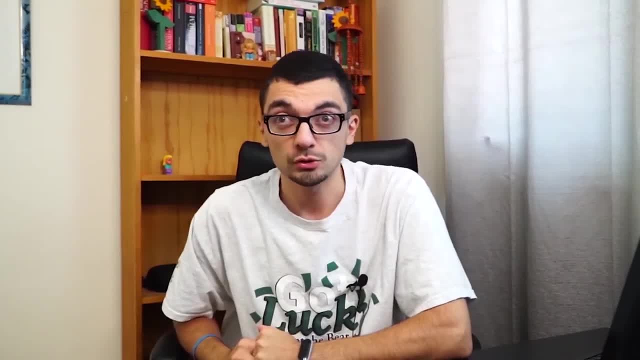 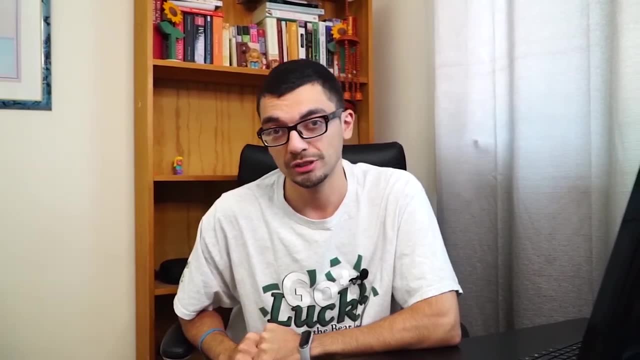 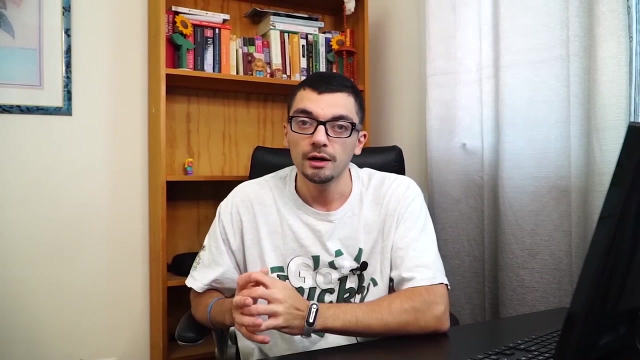 you can choose and you can have benefits: some developments of 2050 years and, as we know that it will be, some global warming issues and ocean acidification and you have to find something reducing these effects and making clean environment. this one is really good because right now almost all countries 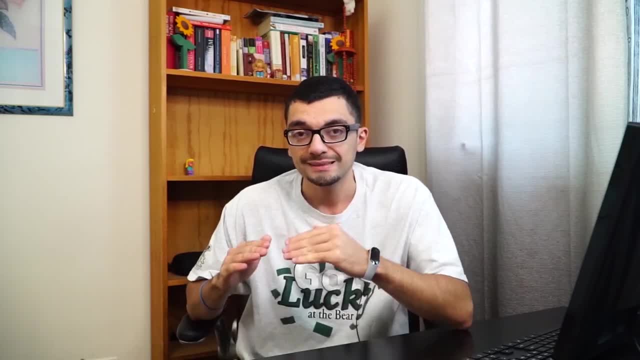 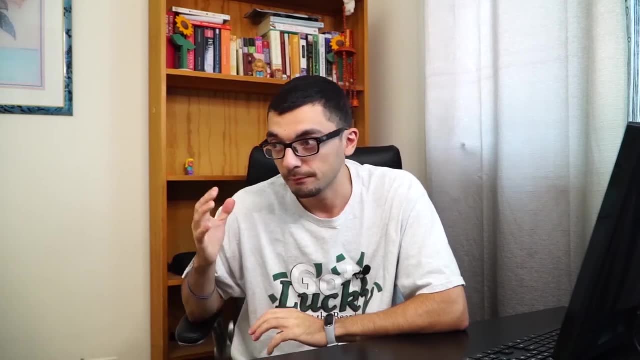 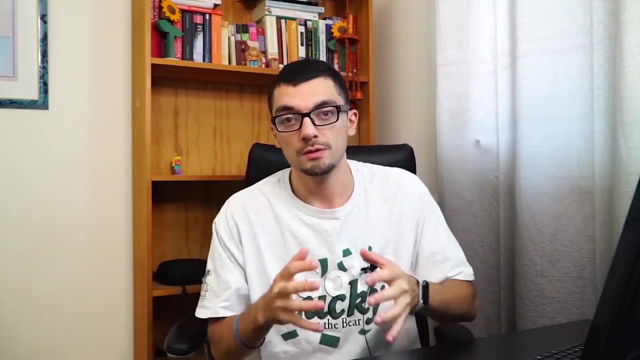 are trying to do their best for minimizing all global warming effects or something shortage of natural sources for 2050, and we know that it will be overpopulation, and we need to keep our environment clean and also save energy. if we are talking about 2050 year developments, we 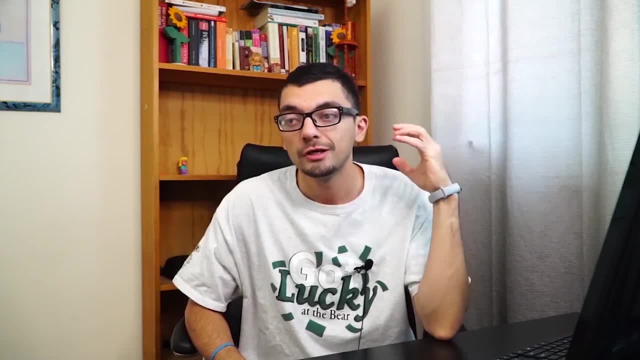 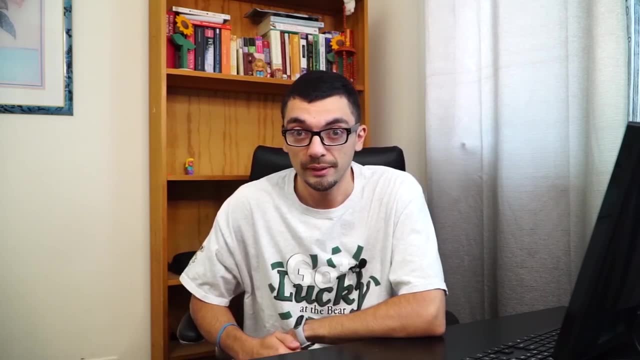 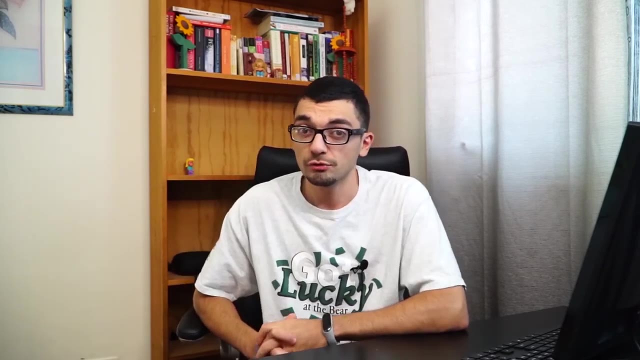 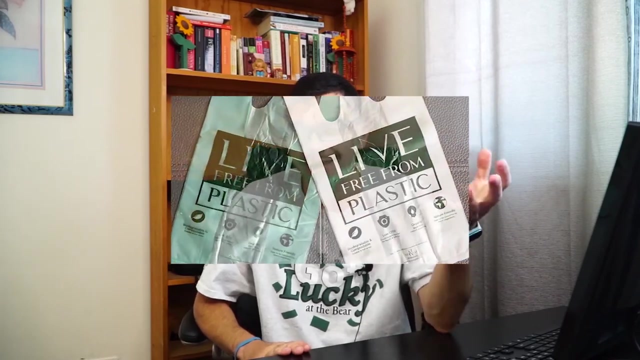 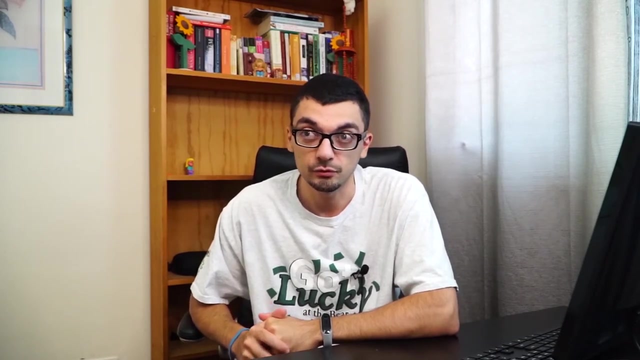 have to take into consideration about food science and technology. yes, because agricultural area also will be impacted. we need to find something really save our agricultural fields: transformation of agricultural waste into biodegradable packaging materials. i can give you the one reference: cassava plants. they are making packaging, biodegradable packaging, from these material, from these food. 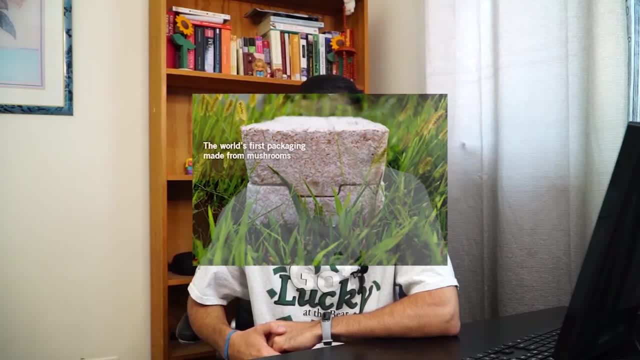 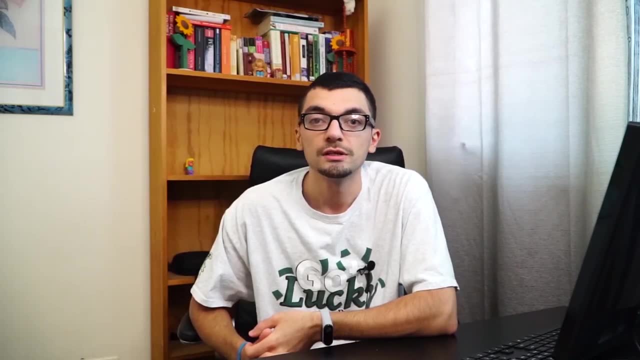 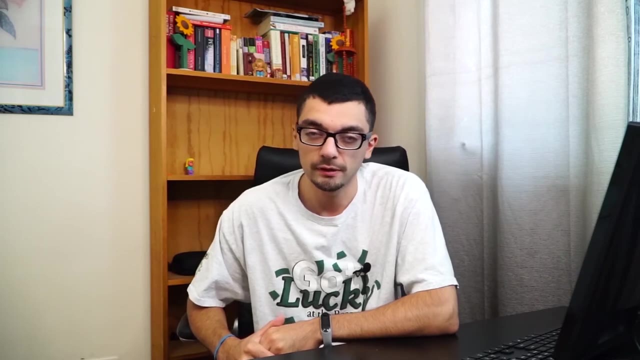 waste and also some mushrooms. they are making carton packaging. it's a really good topic and you can do research, find the best material which is interesting for you. then you can write your teas or scientific publication. another one is seed oil, plant-based oil, as we know that animal based of. 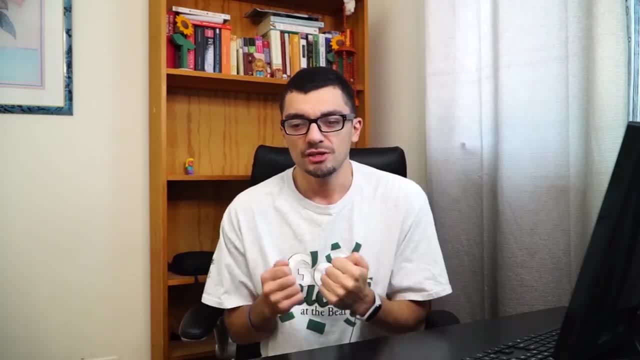 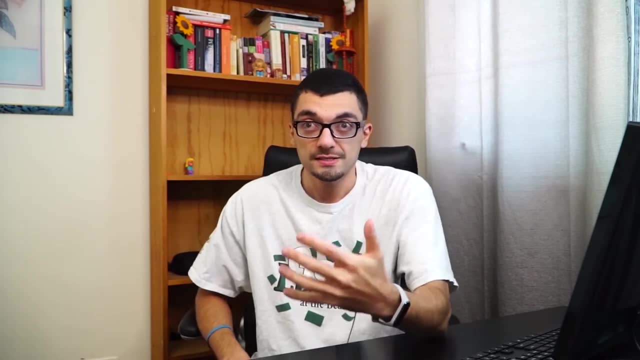 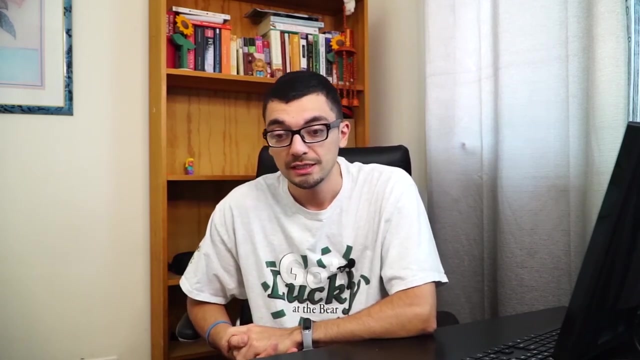 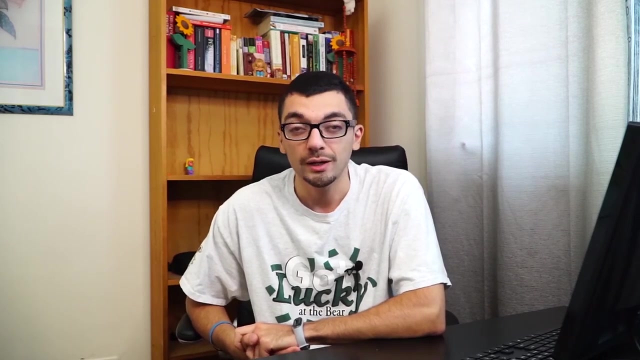 oil or fat are really dangerous for our health and also some people getting diseases because of overusing. you can find something really interesting and production of seed oils, any kind of plant-based oils, and writing the topic will help you to find job in food industry, also agricultural field. 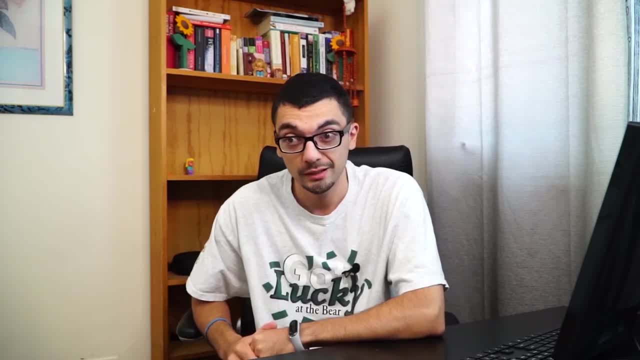 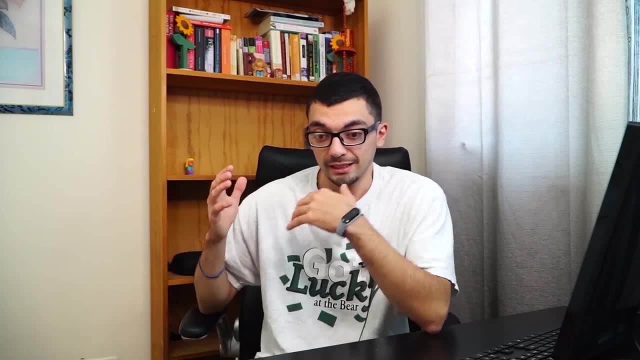 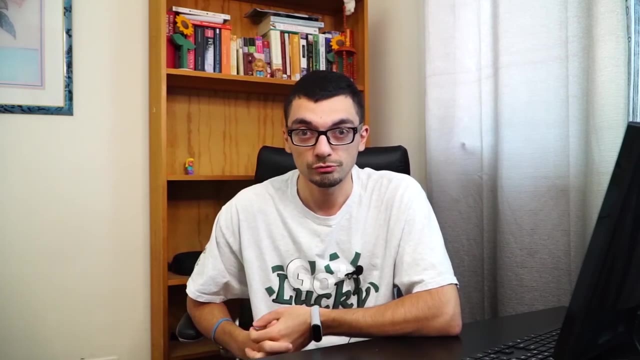 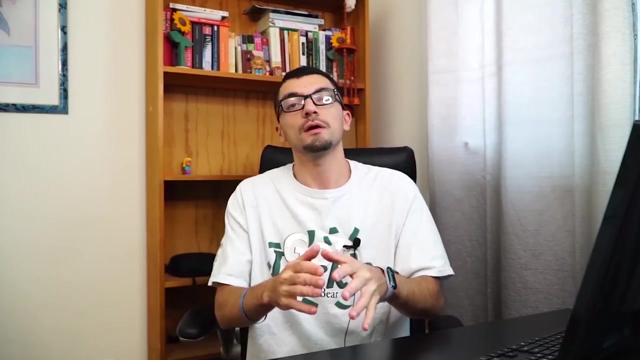 another one. of course, we know that some people are vegan, some people are lactose intolerant, but what you have to know in order to making something available for those people also- lactose-free food production or gluten-free food production, diary-free or these kind of topics- can be really useful if you are familiar of this topic and you are specialized. 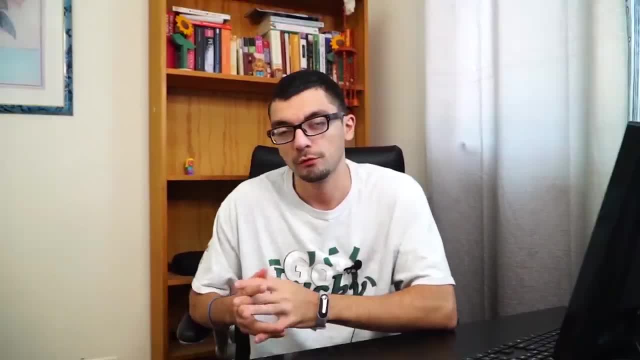 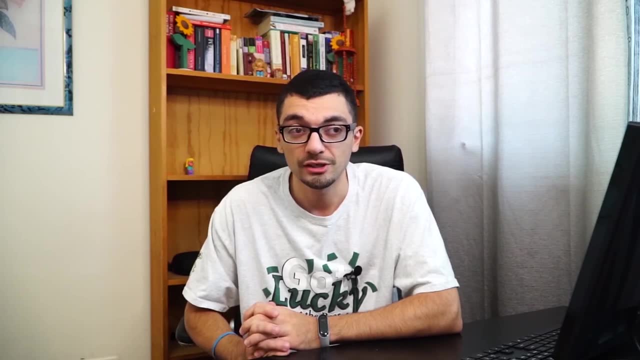 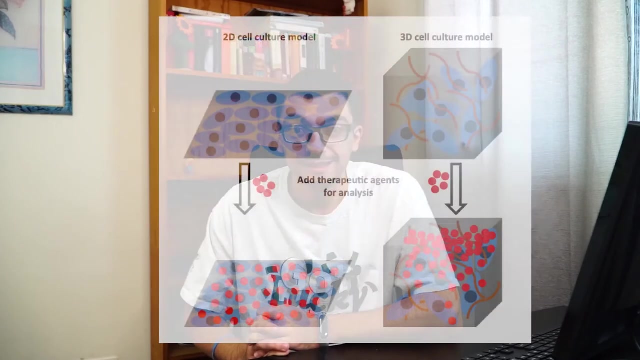 in this area after graduating, where you can work, because which companies are producing alternative sugar foods or vegan foods or lactose-free, diary-free foods, and also the companies which are making 2 or 3D self models. this is really impressive topic and if your field is related to 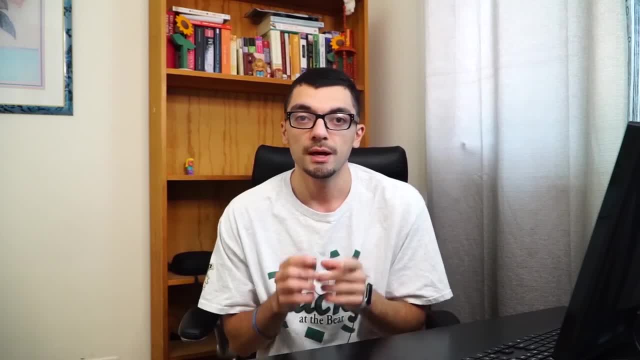 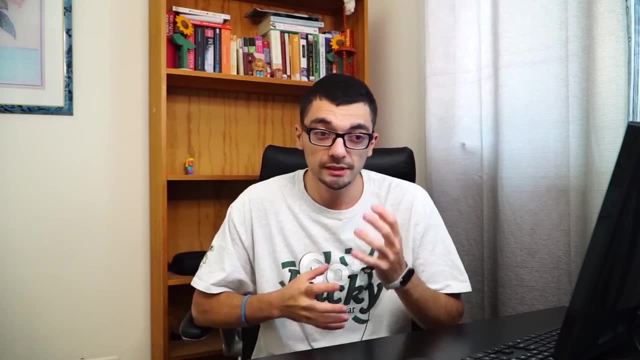 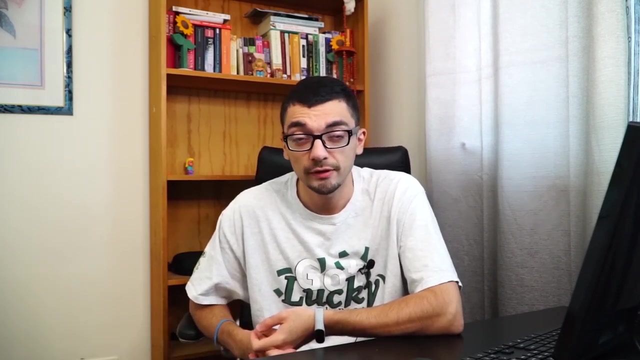 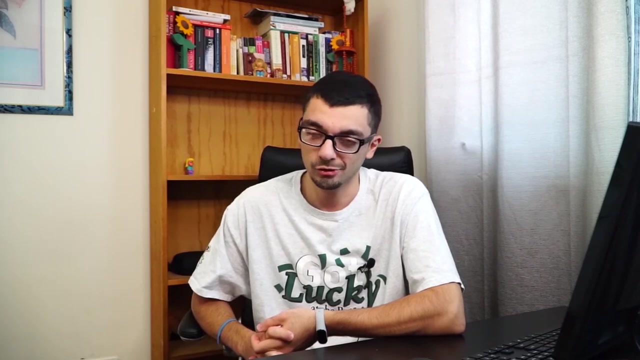 food science and technology. choose these mentioned topics. okay, the fourth one, which is related to toxic industry. explaining of this topic, I can give you information about toxic metal detection, for example, resistive surface acoustic wave to detect toxic metals. this you have to be familiar because it is your area and by doing research you will get more information and another example I can give you. 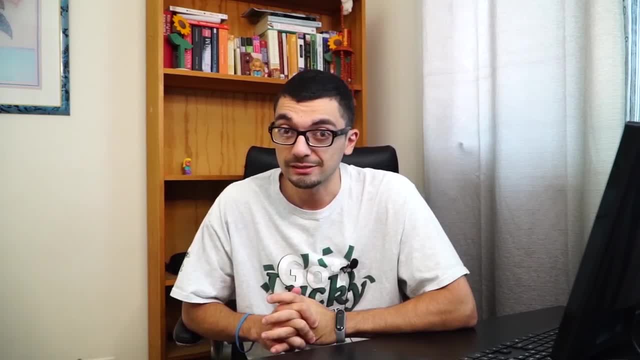 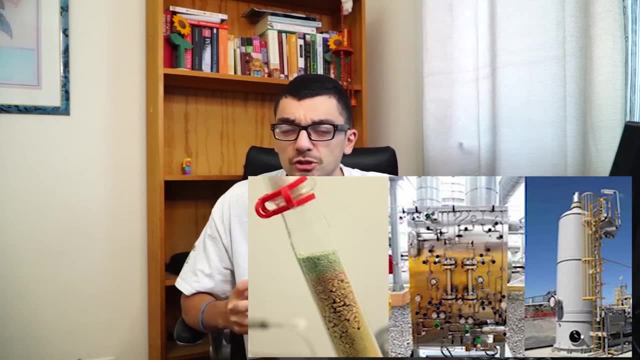 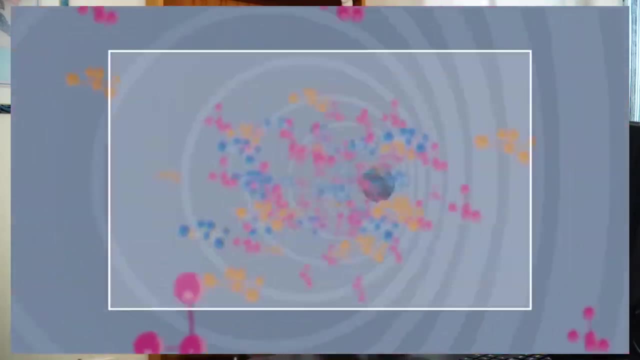 high quality gas sensor testing to detect toxic metals. and last example for toxic metal detection can be mercury removing from natural gas at certain temperature and you have to find which temperature could be really impactful for detecting mercury from natural gas. this is really up to you. you have 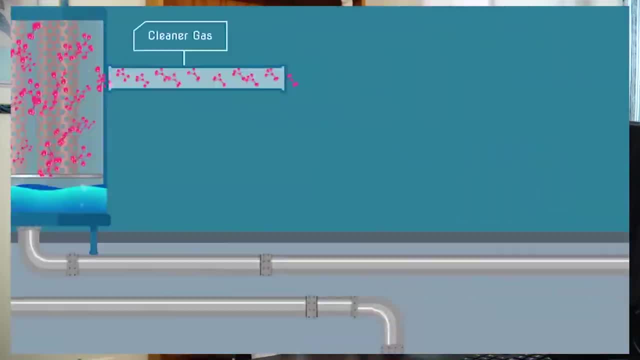 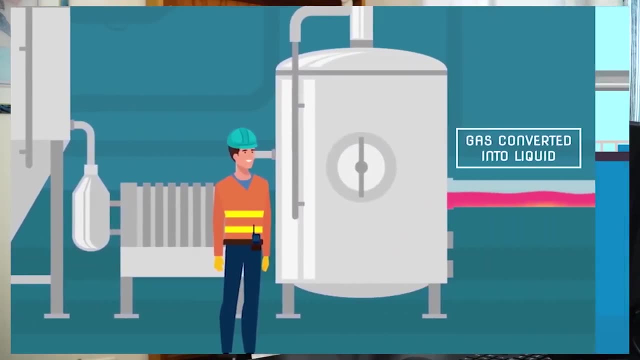 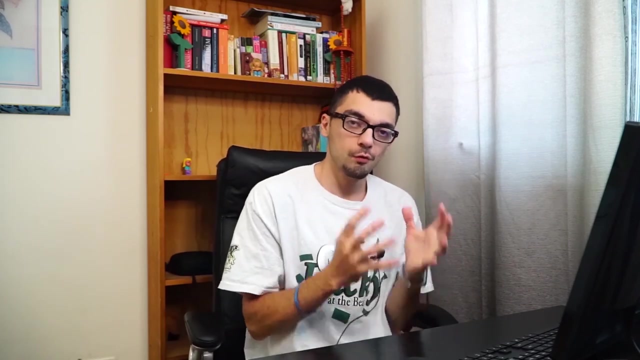 to find the best temperature and also, while doing testing, you will choose the different temperatures. you will successfully write and complete your topic. Okay, the fifth one, Of course. if we are talking about the chemical engineering, we cannot avoid pharmaceutical and nutraceutical industry. 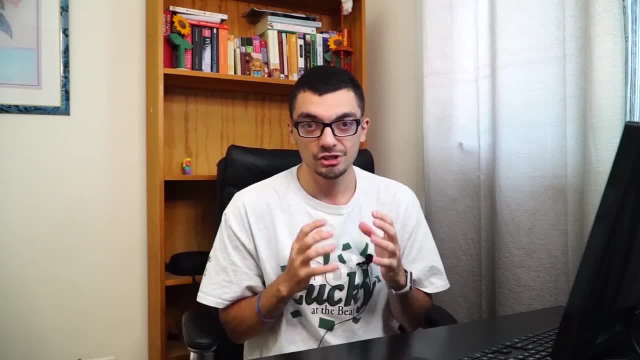 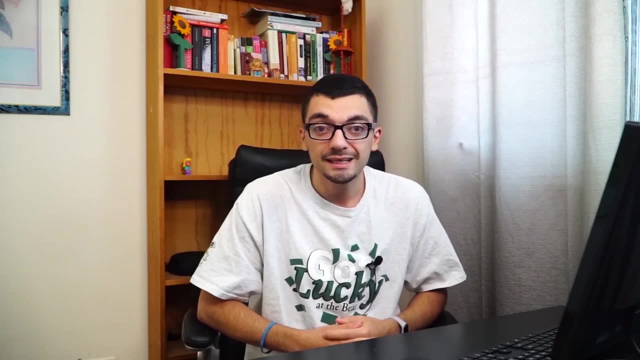 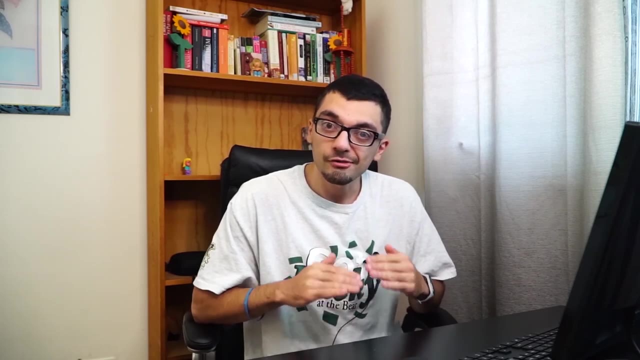 But which topic can be really novel and brilliant ideas for your research? Cancer, Cancer diseases- Yes, this is a mankind disease and still we are discovering something, we are doing some investigation in order to reduce these effects in human or animal bodies, And the novel idea can be: 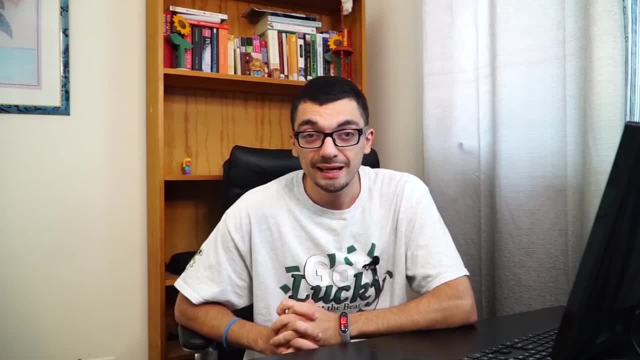 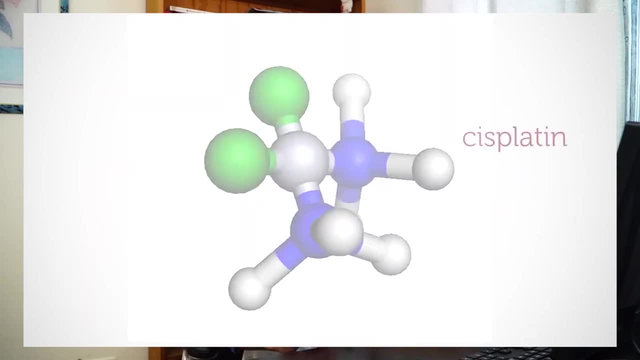 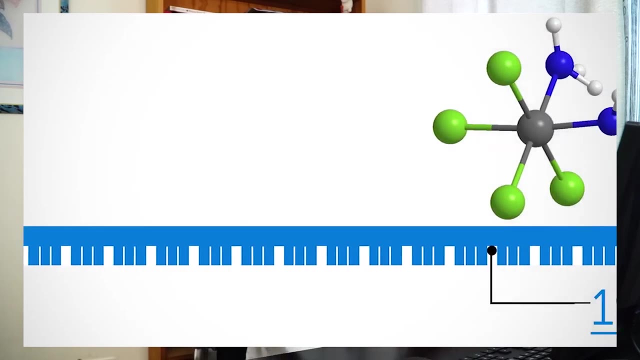 for this area, anti-cancer gold complex which are less toxic for non-cancer cells, or the minimizing of these side effects from non-terminal cancer patients, And that's why these topics can be related to your field and you can choose get benefit in that field. 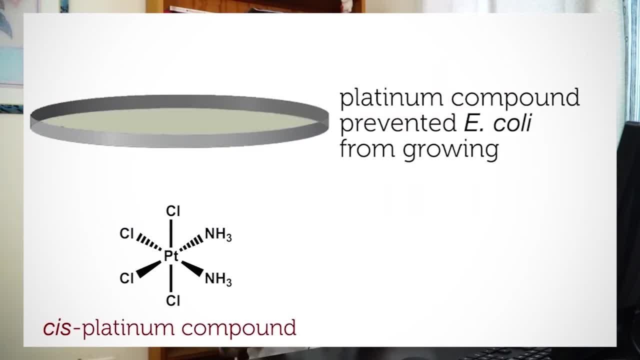 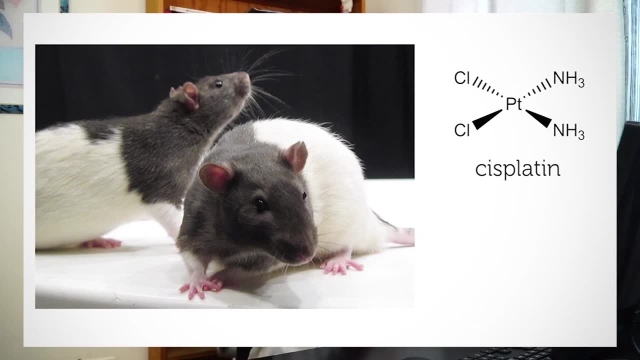 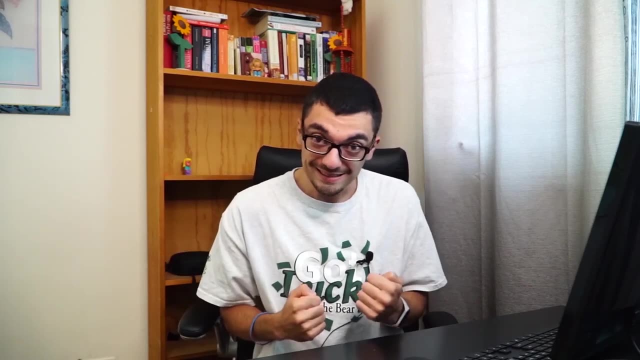 the future and it will really open the doors for you finding jobs easily. i can say easily because outdated topics and we are doing research while studying and after graduating we don't find anything. there is no match between what we studied but what companies are doing right now. if you found, 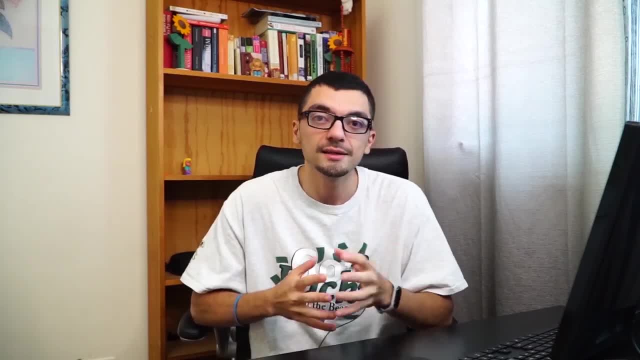 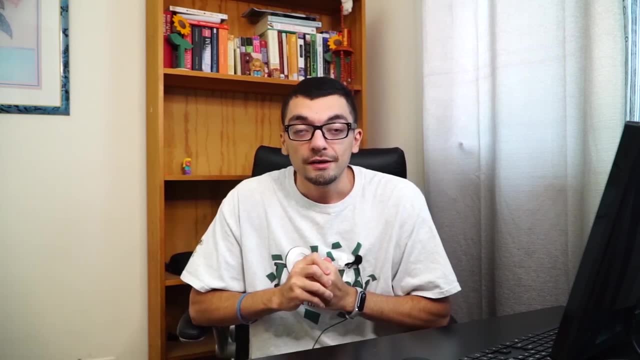 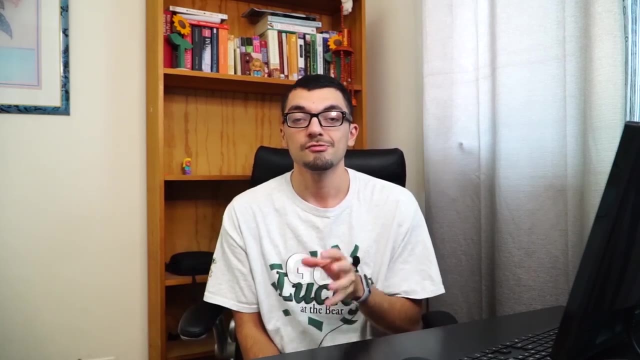 this video really informative and you want me to make a new video about your field? just comment below the next video i will make about your topic. if you enjoyed, hit the button below, subscribe this channel and also give me a thumbs up for helping me to grow with you together, fighting this. 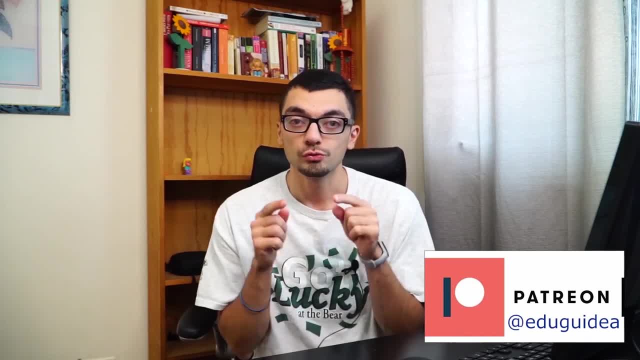 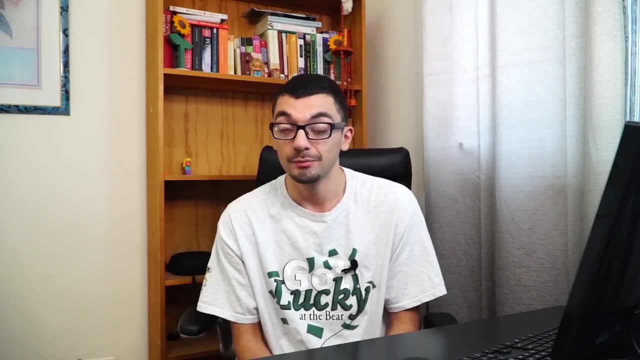 youtube algorithm. it's really important for me you to watch this video while subscribing. take care, good luck in your research fields or future career. bye.